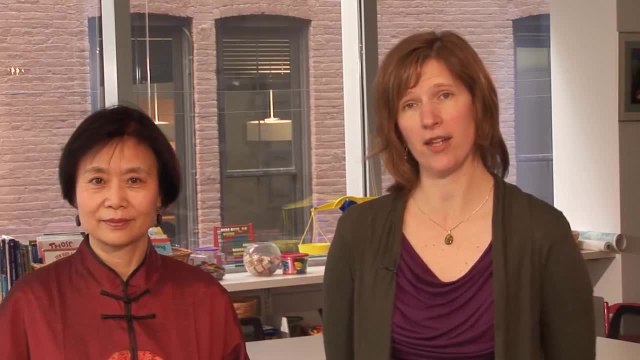 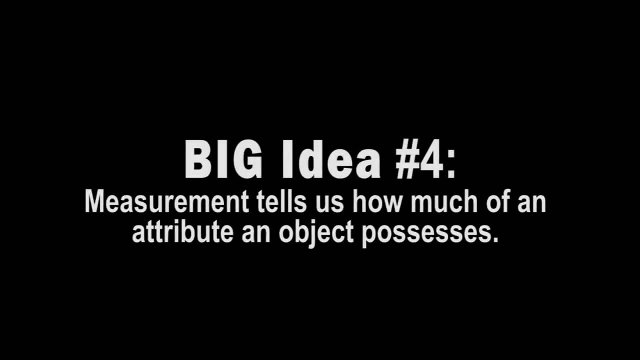 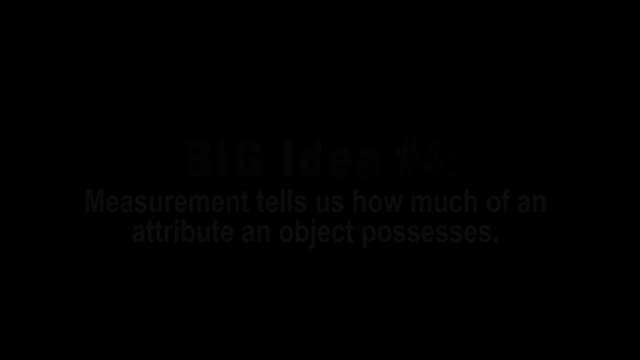 While these five big ideas are not inclusive of all that young children need to learn, they deserve emphasis. Measurement tells us how much of an attribute an object possesses, For instance, length or capacity. How do you guys know when something is big, If it's huge? 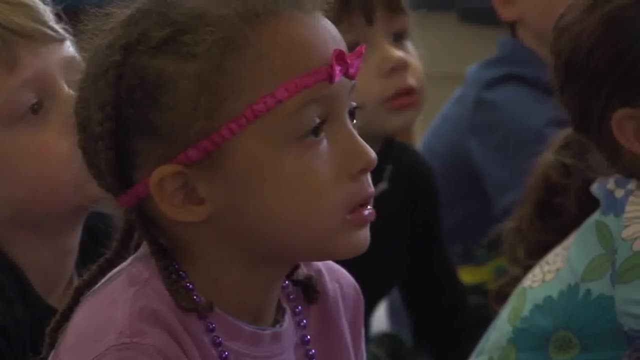 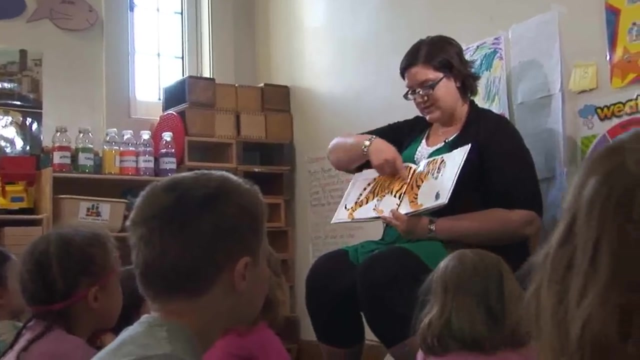 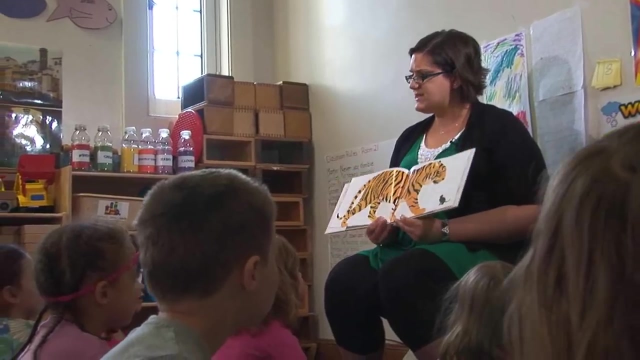 Young children are naturally focused on finding who or what is the biggest. One of the most important concepts for them to learn is that big can mean different things depending on the attribute being considered. They're both cats. They're both cats, And how are they different? 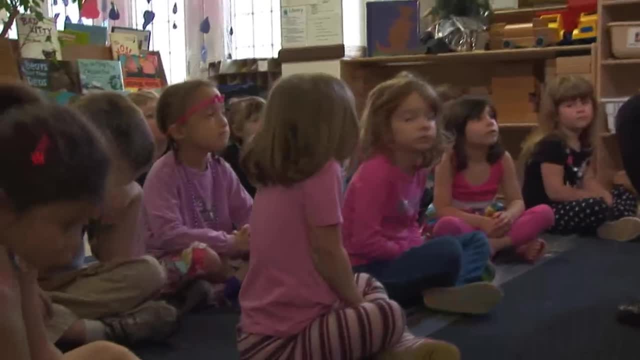 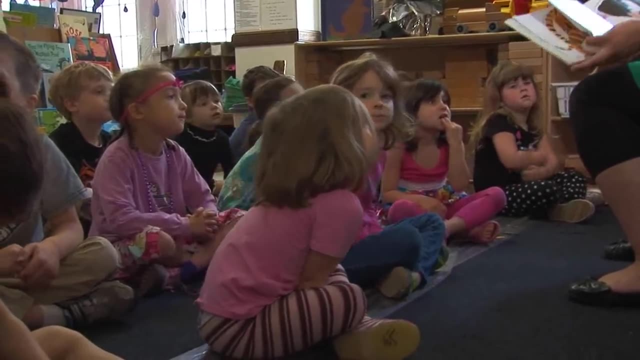 Do they weigh the same? Do you think No? Which one weighs more? The tiger? The tiger, How do you know? it weighs more Because it's bigger. It's a bigger animal. The first requirement of measuring is deciding what attribute to measure. 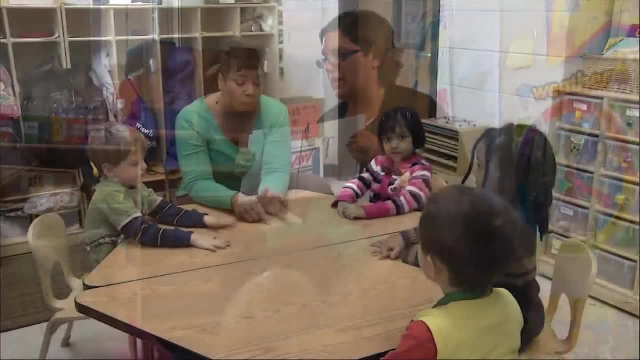 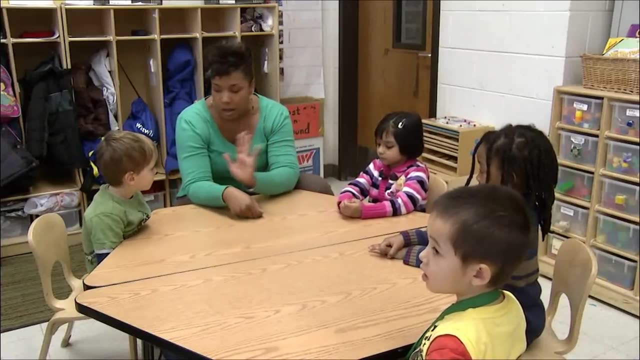 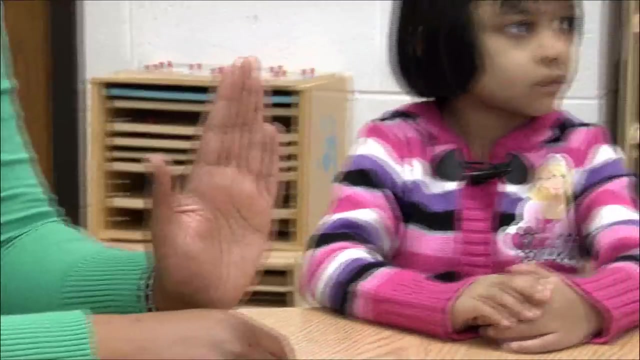 What kind of big are we talking about? We're going to try to find something that is the same size as our hand, the same length as our hand. How would we know how to measure something that's the same length as our hand? Length is the easiest measurable attribute for children to consider. 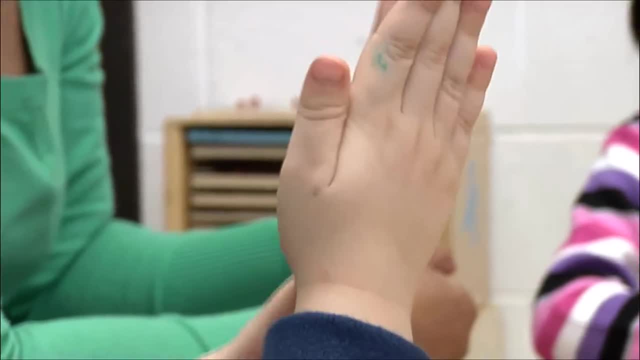 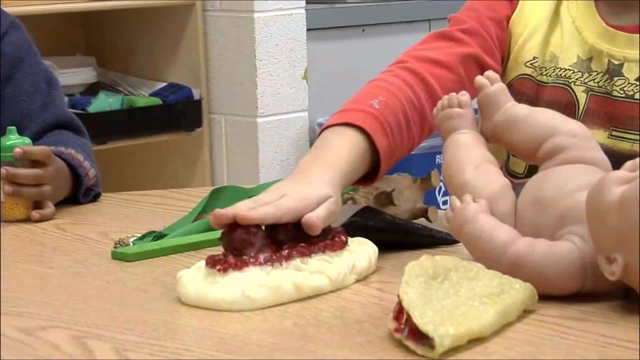 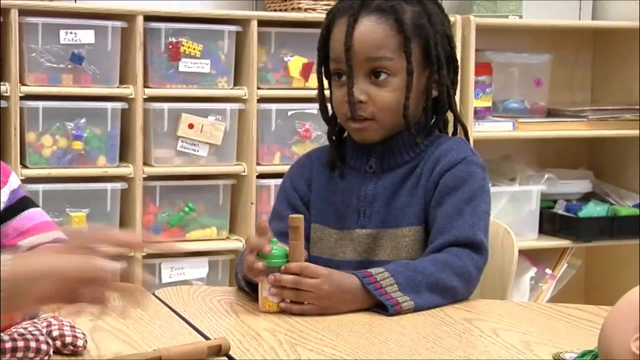 Even very young children are sensitive to differences in lengths, although they can easily be misled by their perceptions. You think With experience they realize that measurement requires them to compare things directly to see what is bigger and what is smaller, Small, Small. It's shorter than your longer. one right. 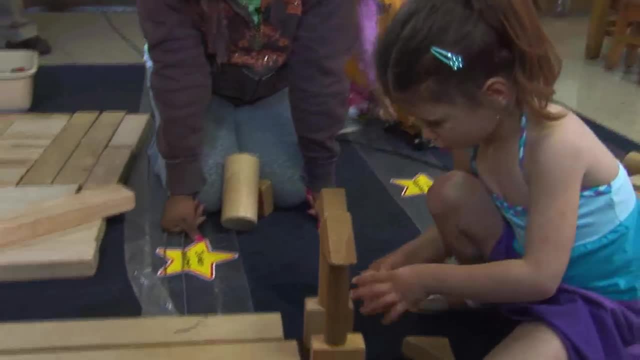 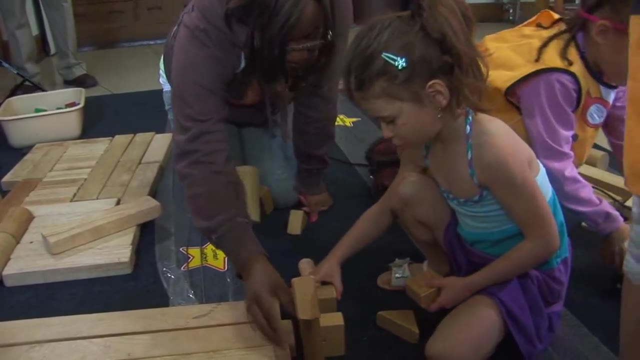 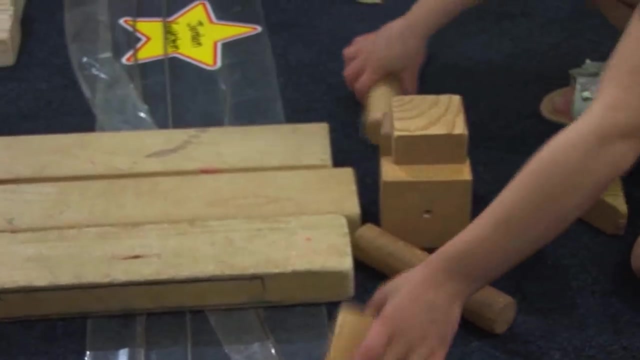 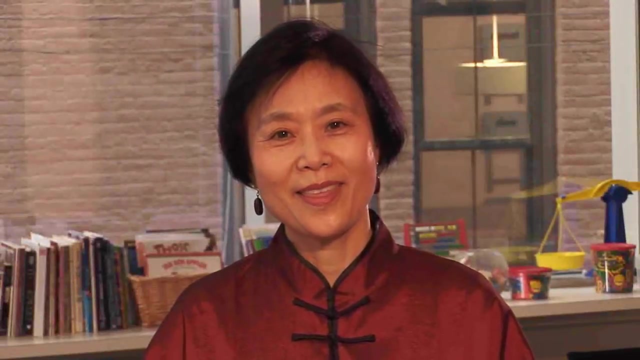 A variety of experiences. comparing objects enables children to become more precise in their language. Longer, wider, narrower They begin to understand that these measurement concepts exist only in relationships between objects and not in the objects themselves. When thinking about young children and early math in schools, 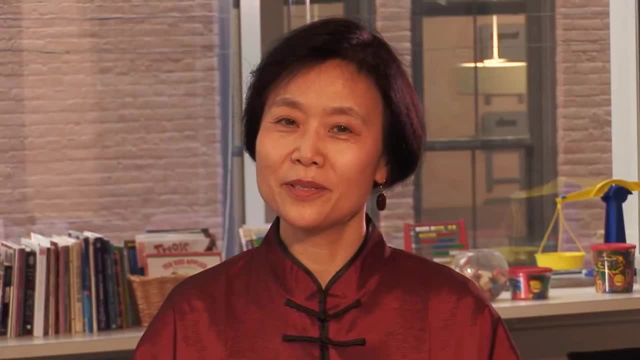 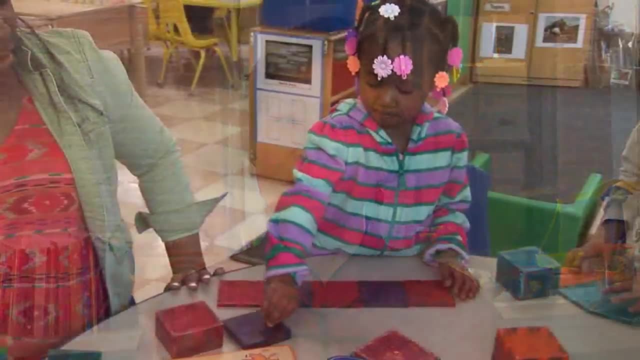 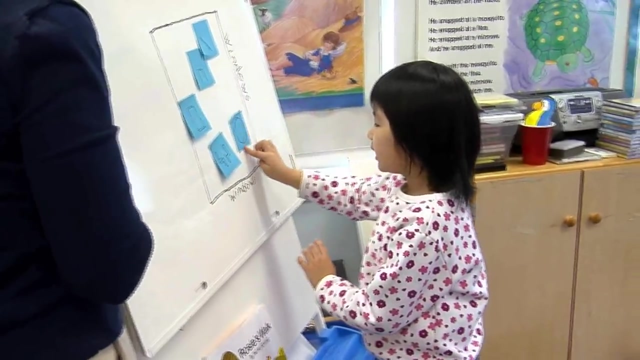 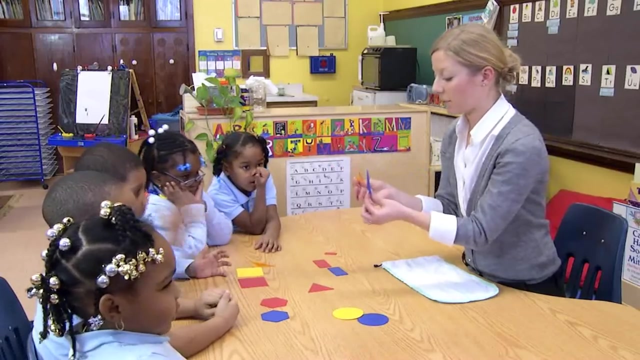 there are three messages we would like you to take away from this film. The first is about children. Young children are eager, curious and capable of learning math. The second is about the teacher. Teacher competence in teaching mathematics depends on understanding the big ideas. 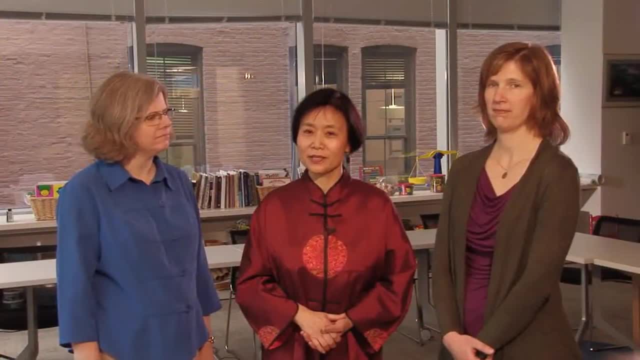 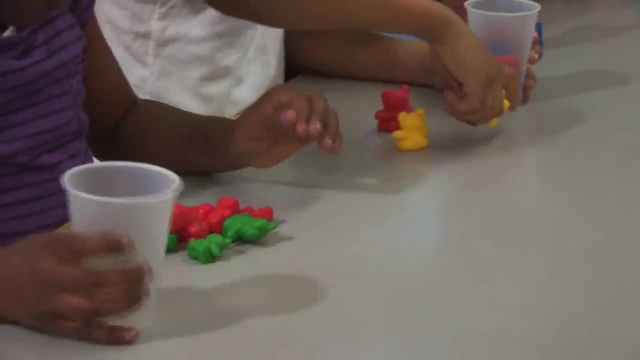 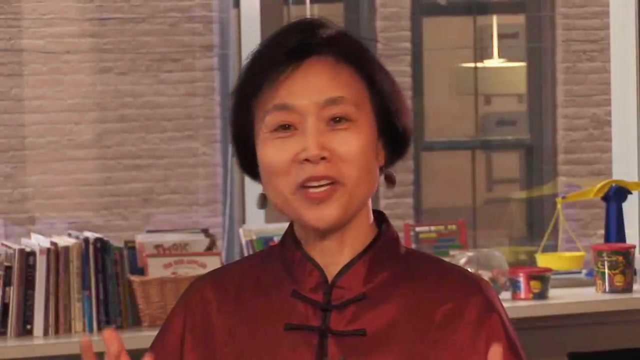 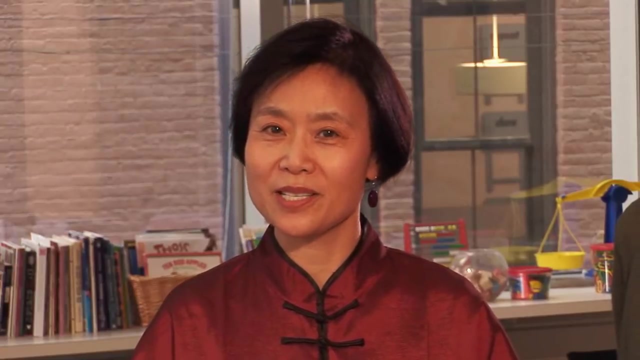 The third is about children. The fourth is about classrooms. Quality early math learning in the classroom requires both intentional teaching and mathematizing children's daily experiences. We trust you will find it rewarding to provide rich math learning experiences to your students because you are helping them build foundations. 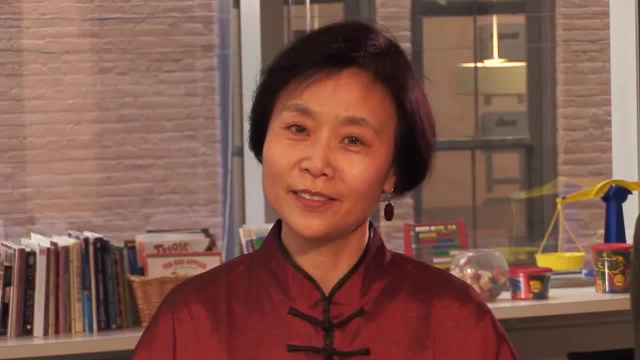 for further math and lifelong learning. 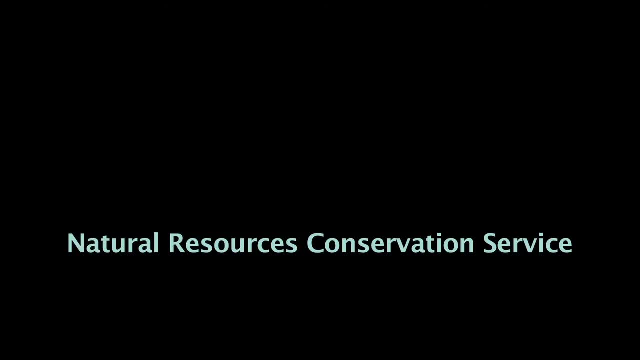 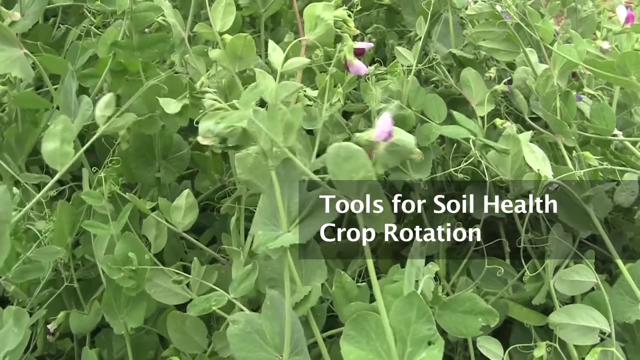 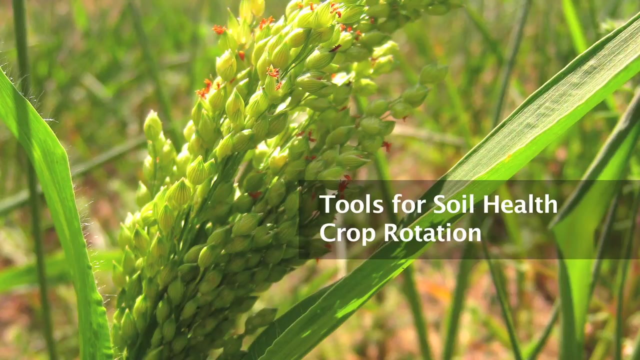 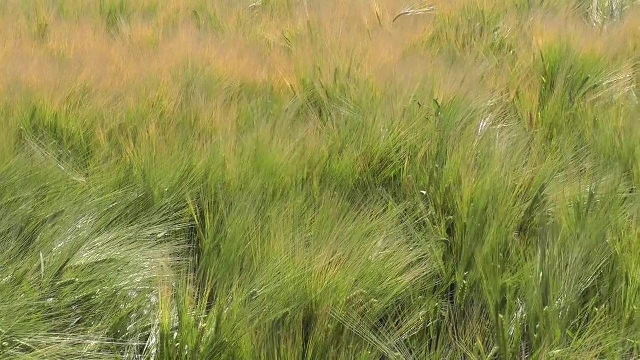 This segment in the Soil Health, a Montana Perspective video series will discuss one of the tools that agricultural producers can use to improve soil health. This tool is crop rotation. A conservation crop rotation increases crop diversity by growing different types of crops in a planned cropping sequence. There are four types of crops- cool season grasses, for example. 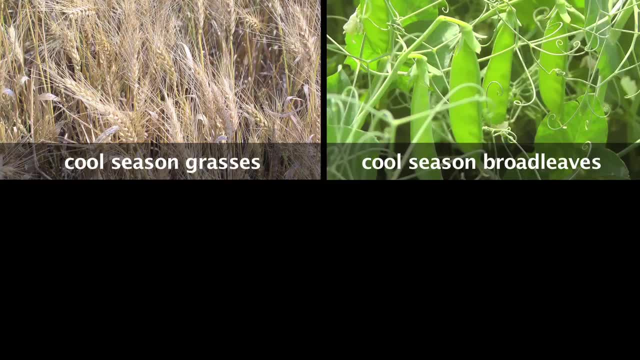 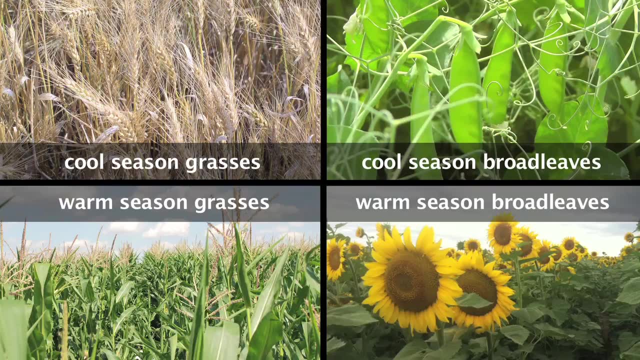 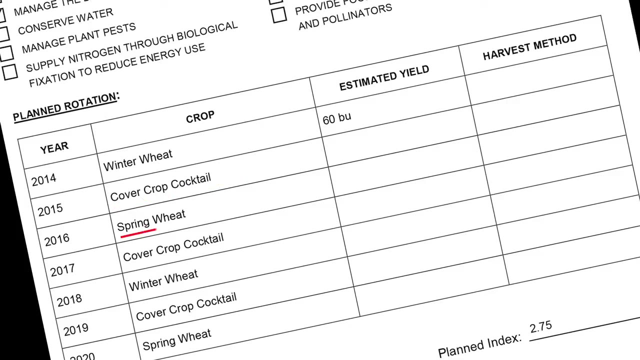 small grains: cool season broadleaves, for example peas and flax. warm season grasses, for example corn and millet, and warm season broadleaves, for example soybeans and sunflowers. For a successful diverse rotation, it is important to have at least two different crop types in a 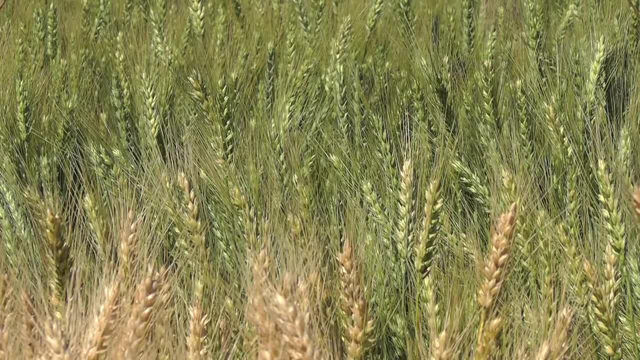 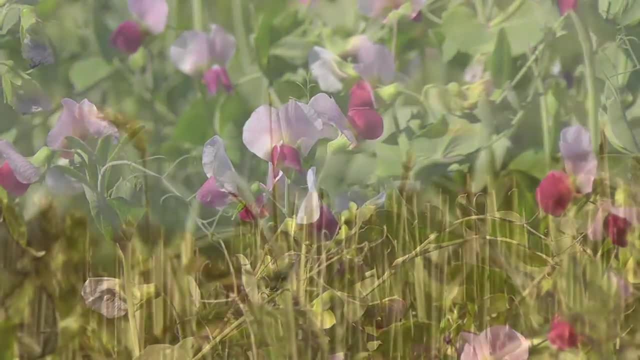 field before you come back to your original crop. For example, if you planted wheat, you might want to plant corn and peas in the subsequent years before you went back into wheat. In this rotation, you would have three crop types represented. This increased diversity can help reduce disease. 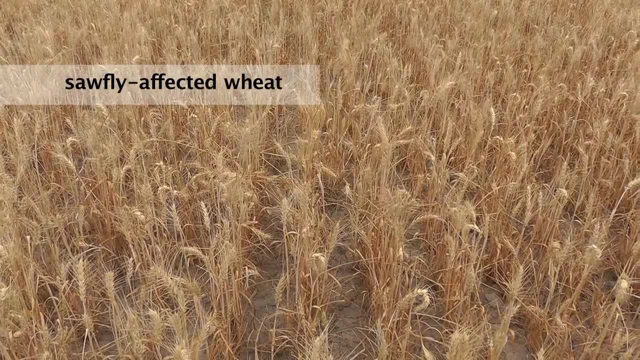 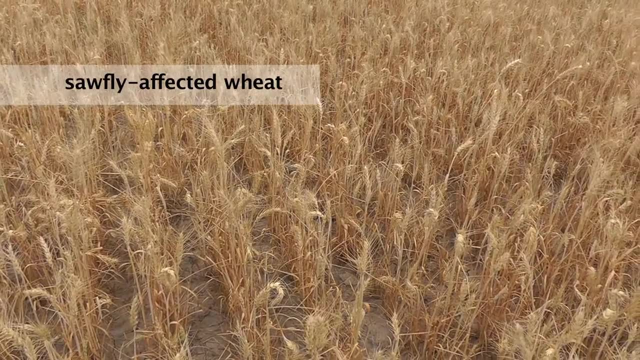 and pest pressures by breaking up disease and pest cycles and or allowing for the use of different disease and pest control methods. that might not be possible in your regular cropping system. Crop rotation can help with nutrient management as well. Legumes can be used in the rotation to